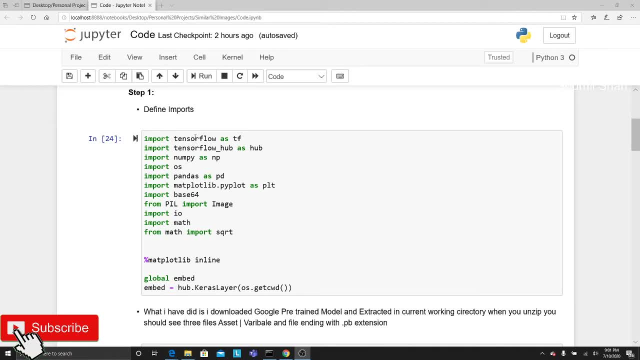 So the following are the list of imports that we need to do, That is, TensorFlow, TensorFlow, Hub, NumPy, OS, Pandas, Matplotlib, Base64, PIL, IOMath and SQRT from the math And make sure that the TensorFlow version that you're using is 2.0.. Second, we need to create an embed, a global variable called as embed, And basically we are going to use hubkheraslayer and osgetcwd means get the machine learning model, which is basically downloaded on my current machine learning model. So that's the list of imports that we need to do. 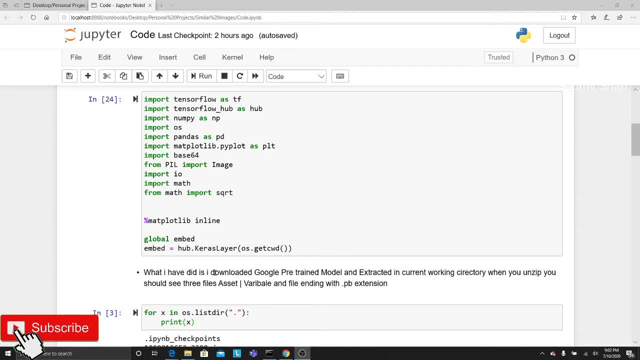 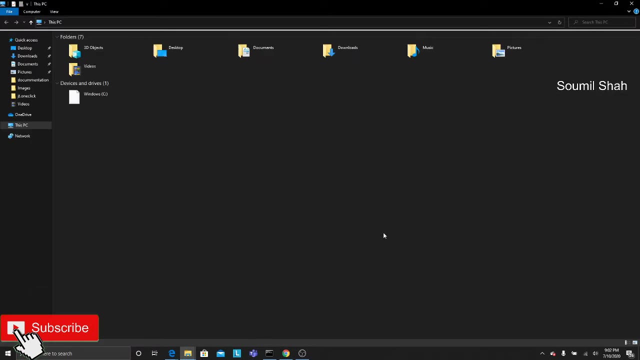 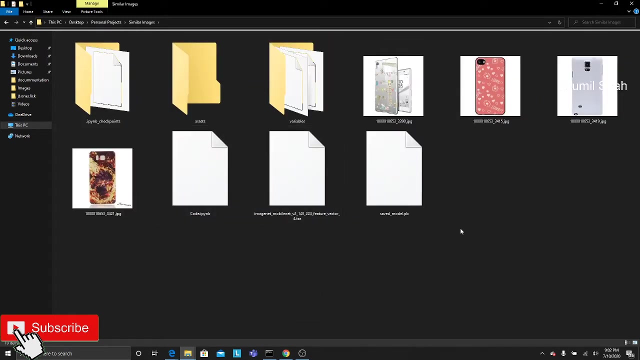 So I have a note here: When you download the machine learning model and you extract it, it's going to be a zip file. So when you unzip it you would get three files. That is the variable folder. Then you would have a folder call as assets And then you would have a folder call as some saved pb file, Basically file extending with pb. Let me actually show you So this makes sense. So here you can see saved model, pb variable and assets. 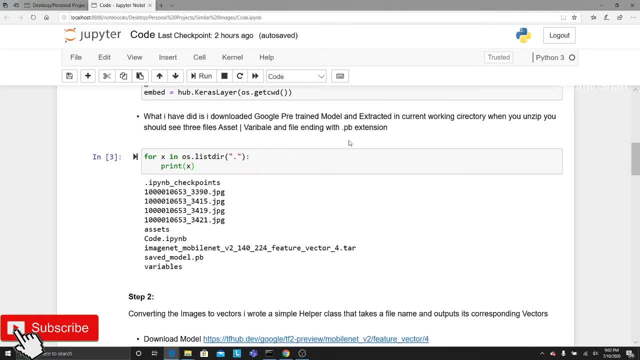 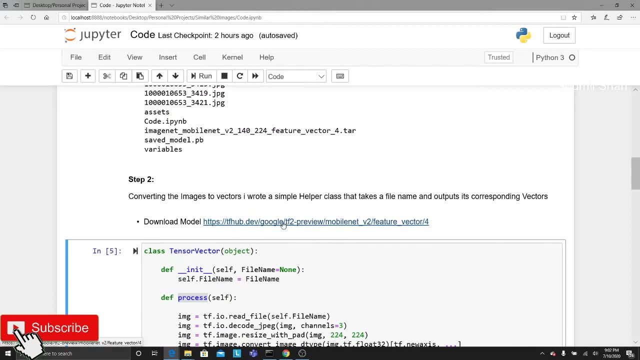 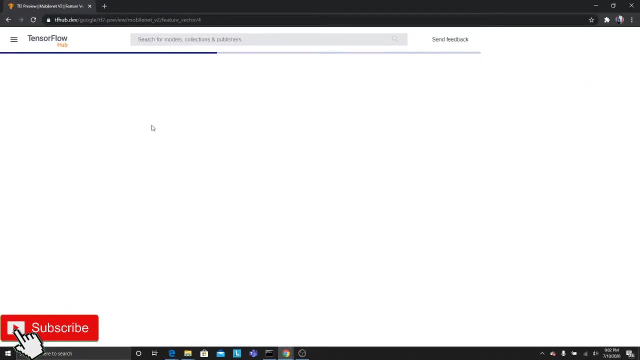 Now, don't worry, everything is there. the links from where you can download these are right here. so from the tensorflow website, or tensorflow hub website, you can download it. so if you go to this website, this is the google's pre-trained model that i'm about to show you. so, kp. so here you can see. mobile net v2. 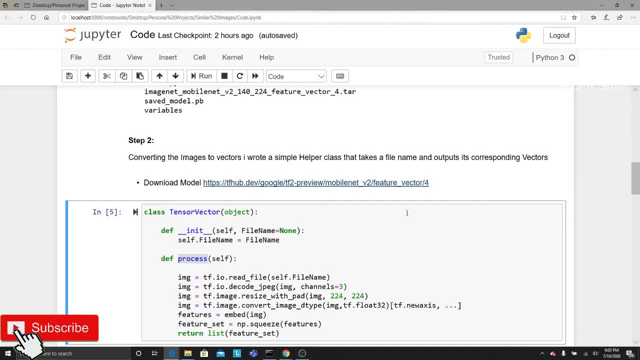 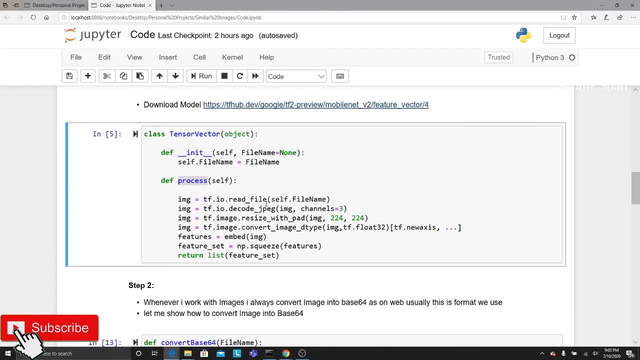 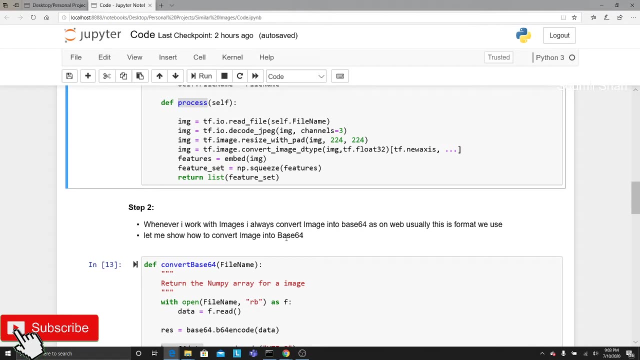 feature vector. this is the architecture by google, so it's a pre-trained model which basically gives you word embedding. i wrote a small class, or a helper class, which takes an image and basically converts into a vector. okay, so let me show you. whenever i work with images, i always have a very 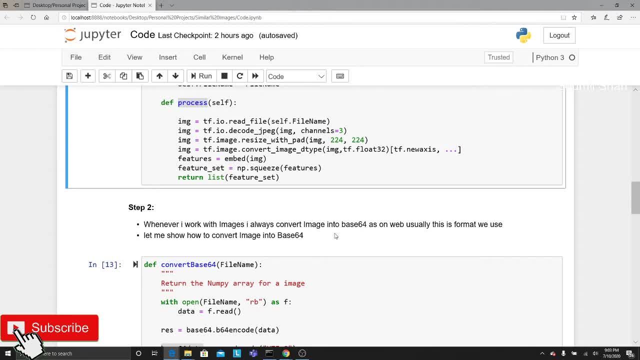 good idea. or i would say i have always a habit of converting those image into a base 64, because whenever you want to display it on our website or do any kind of image manipulation, you can always retrieve images from base 64, rather than having a binary object or a blob object which consumes a 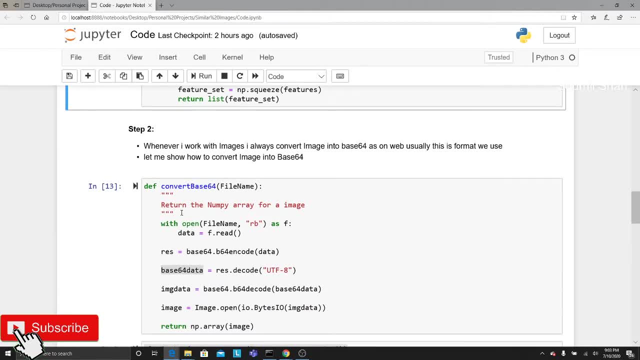 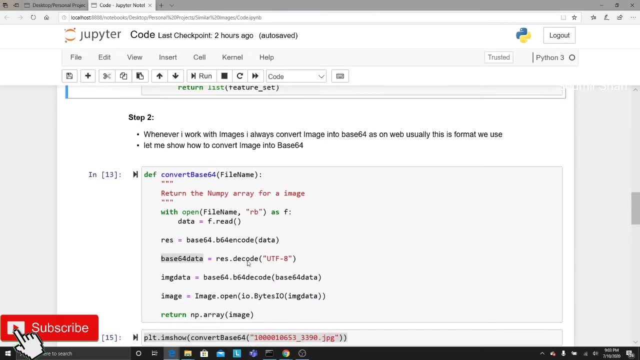 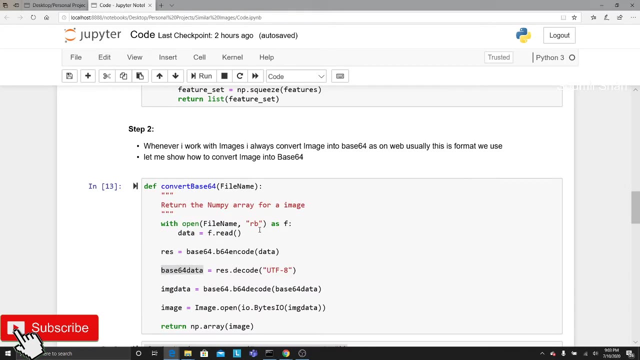 lot more in size. so basically here is a simple class. i just wanted to show you it reads the current file. so in this case i'm reading a file called as 100 on my computer. here you can see oslisters. so all i do is guys. here is basically i read the file as a binary, then basically convert that by a. 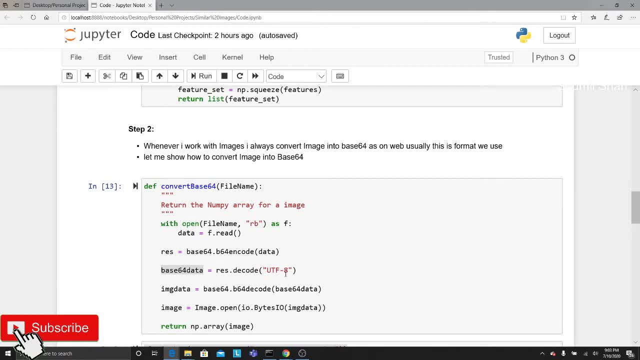 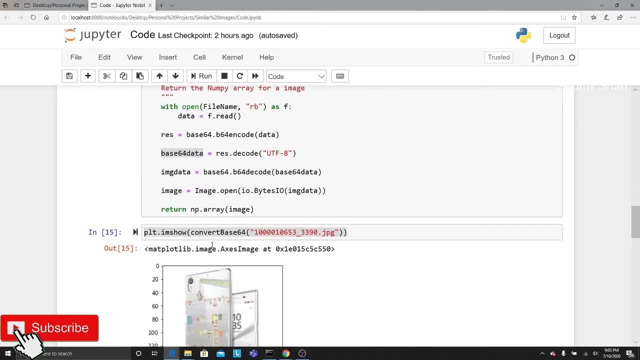 blob object into a base64 and then i decode the base64 bytes into a base64 string, then i convert that into a numpy array. converting that image into a numpy array, now to display, i just say pltimshow. so here, basically, i just want to show you that this is the image, right, and i'm going to take one. 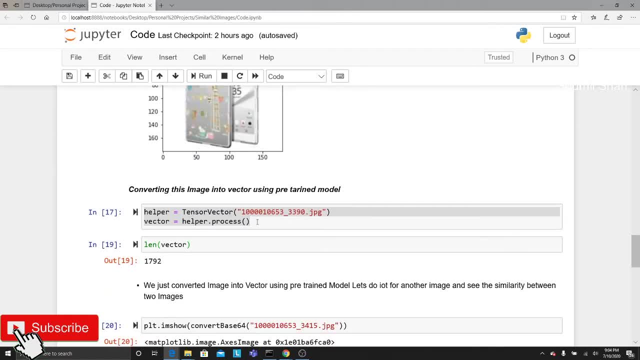 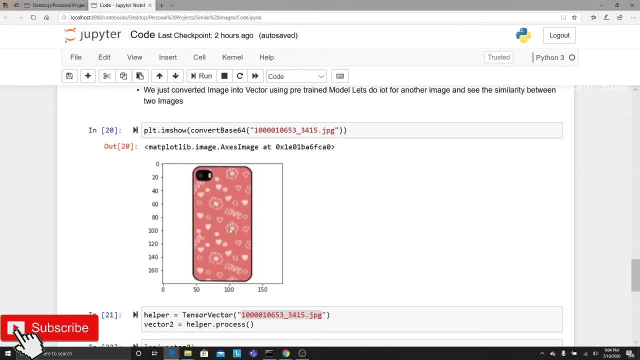 and then we will perform the similarity search algorithm. for example, i took one more image and i display, so you can see. both the images are of mobile phone cover, so we want to see how similar these two images are. so what we will do is basically convert this image into vectors, using 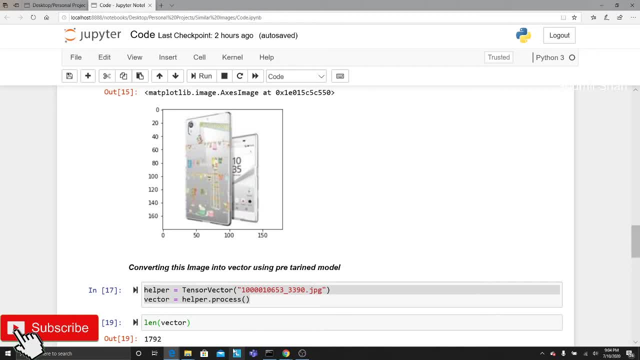 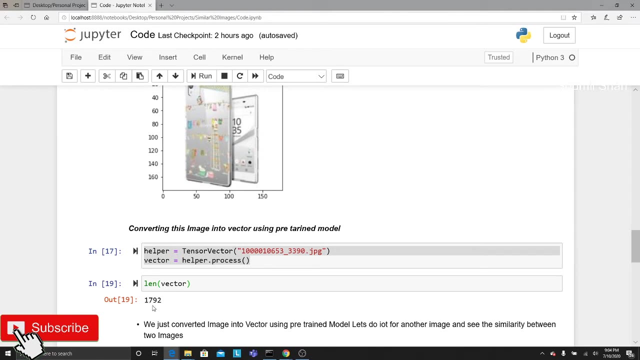 google's machine learning, basically pre-trained ml model, as i said. so i created a class, so i created an instance of a class tensor vector. i pass in the file name, then i say dot process. this will basically give me the vector, which is basically a single array of 1792 items in that array. similarly for 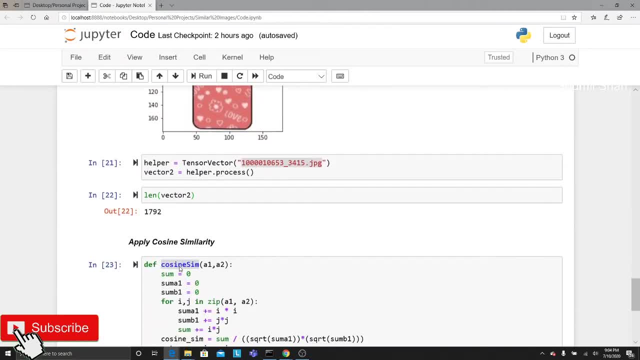 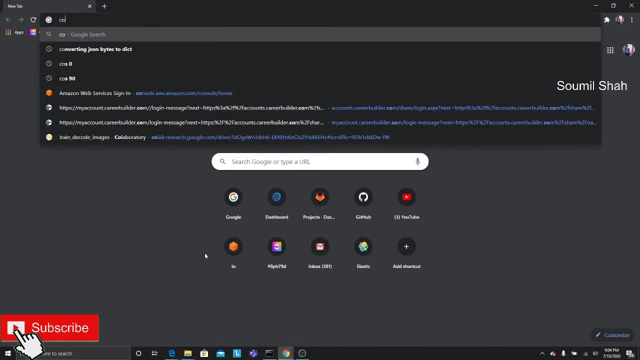 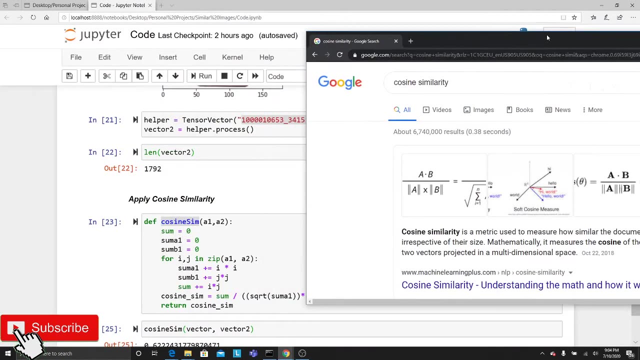 this image. i also convert that into an array here. you can see now i apply the cosine similarity algorithm. so i have talked a lot about cosine similarity algorithm in my videos, in my machine learning videos, so i can't i can again show you once again. i just want to show you the formula. 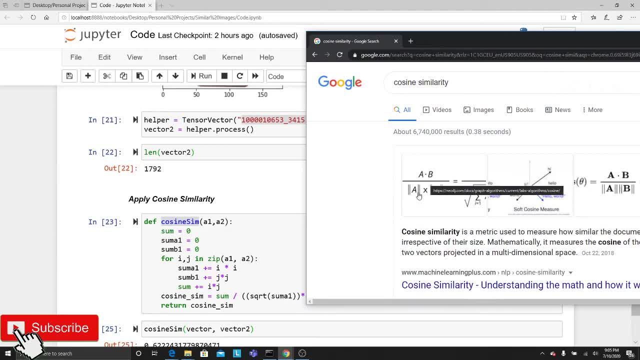 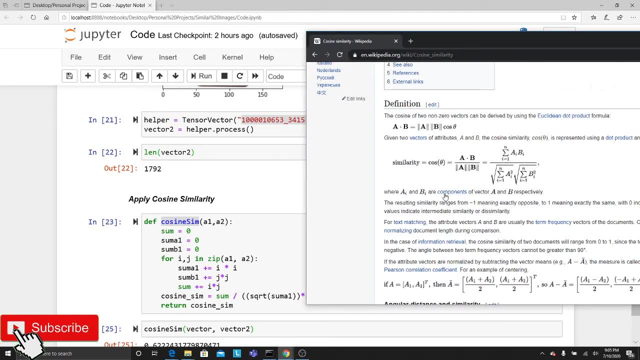 then you can of course verify that. so the formula says a dot b into a cross. what does that mean? if you see on the wikipedia, it's pretty easy, you can mimic it. so from i is equal to 1 to n, that is, from the length of the array sum of a1. so you want to compute first. 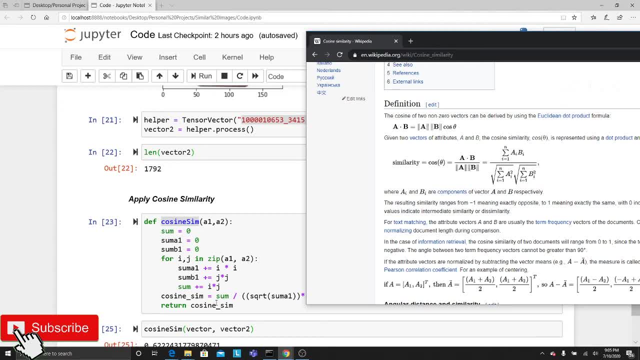 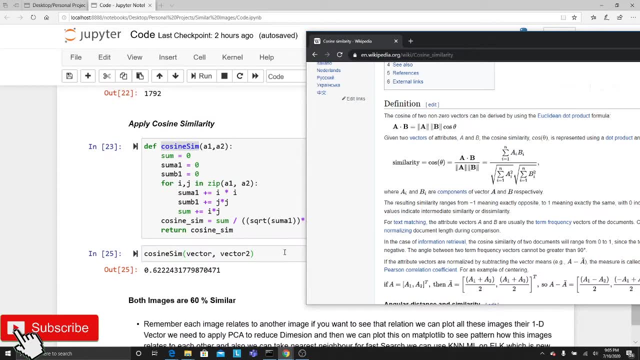 element into first, second flick. you know you want to compute this formula, so basically i just coded this formula. whatever it is given here, summation is basically a loop, so this is what i did. so now, when you pass the, both the vectors, when you convert these images into vector and you pass 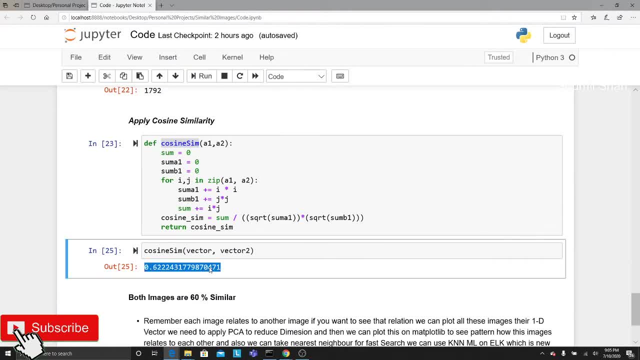 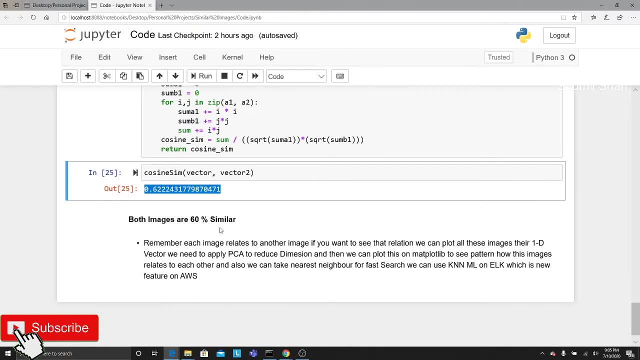 it to cosine similarity. you can see these two images are 60 percent similar and it makes sense because these both, both images- are of mobile phone right. i have added so many comments so you can read it or read this. remember each image relates to one another. if you want to see the relation, 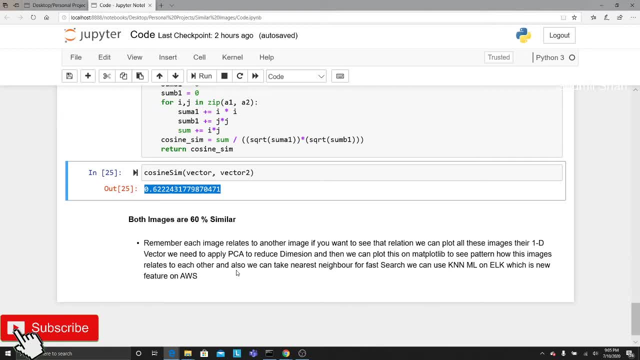 between these images or products. what you can do is basically you can convert this image into vectors, apply pca to reduce the dimensionality and then do a plot. in that way, you can see in 2d, two-dimensional space how this image are related to each other, how close or how far they are, and based on then, if you, if you don't want to do the 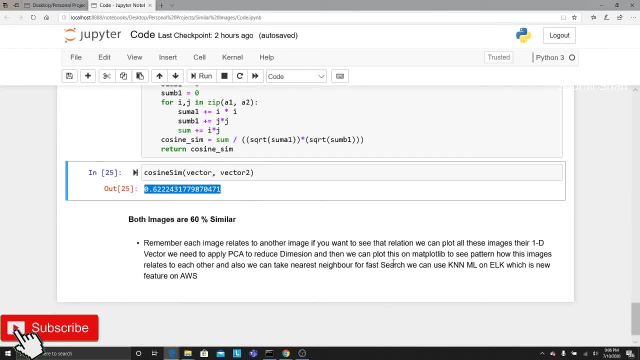 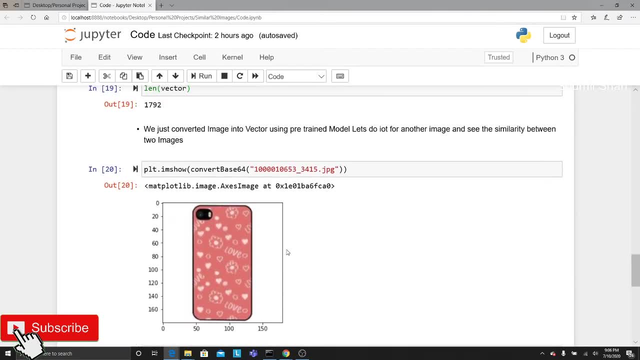 cosine similarity. you can apply a knn algorithm on it so you can take the nearest algorithm and you can get the similar images from that. this type of approach, as i said, is used uh extensively in basically a search engine. so i in my first video- that is the part one i talked about how you can. 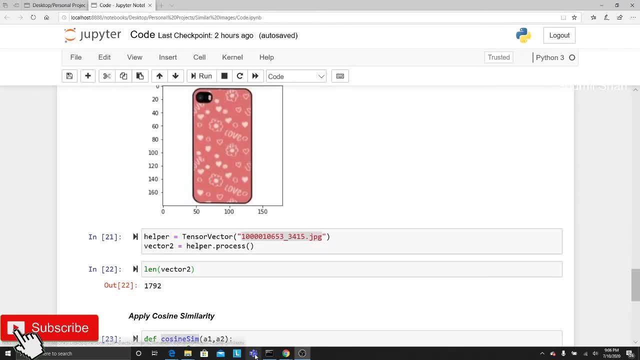 develop an efficient search engine using uh, elastic search. so you convert all of these into a vector and then you upload all of this into a vector. as you guys can see, thecion is very similar and this type of approach is very similar. so you can just use the kind of method in which you use. 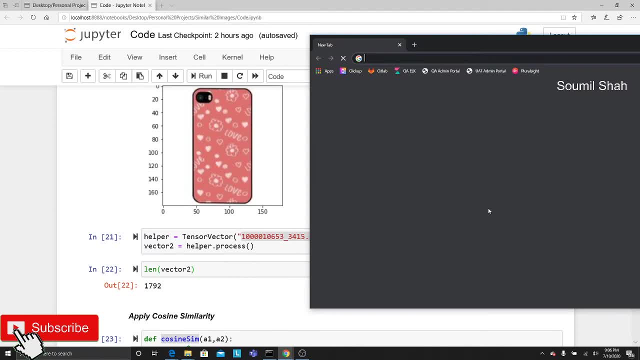 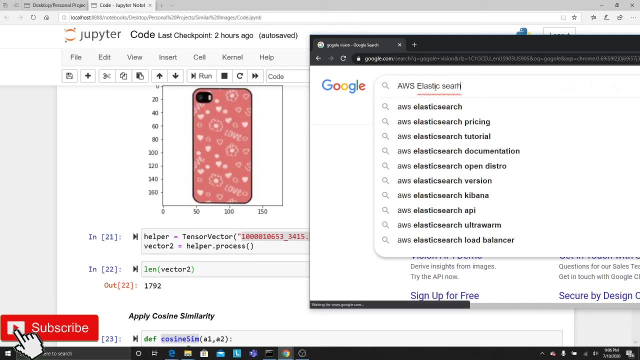 and you convert all of this into a vector and then you upload all of these two images into a vector and vector into elastic search. for those people who don't know about elk, let me just show you something. elastic search on aws: aws, so researchly, sorry, my bad. recently they released basically a. 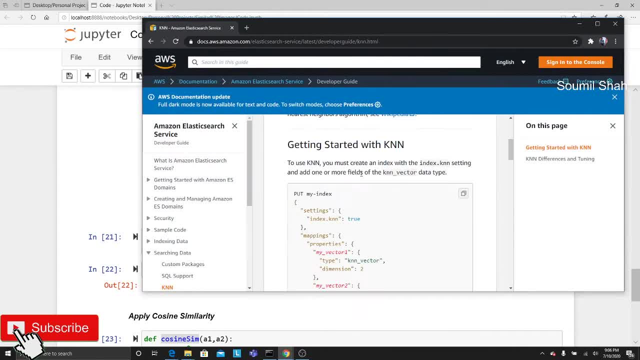 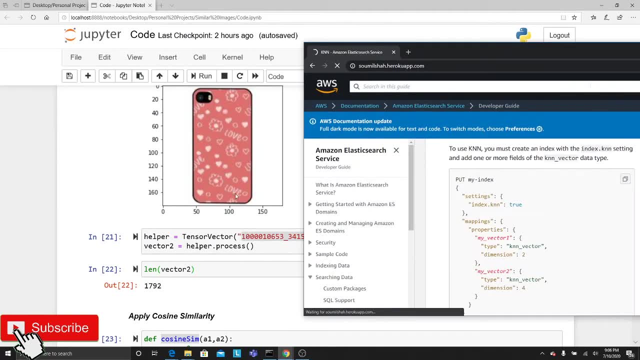 knn version so you can perform machine learning on elastic search, and i also did. i also created a very nice blog article on that. i think it's very informative. i would highly recommend you to watch that blog as well, if you are interested, because when you, if you have like more than 10,000- 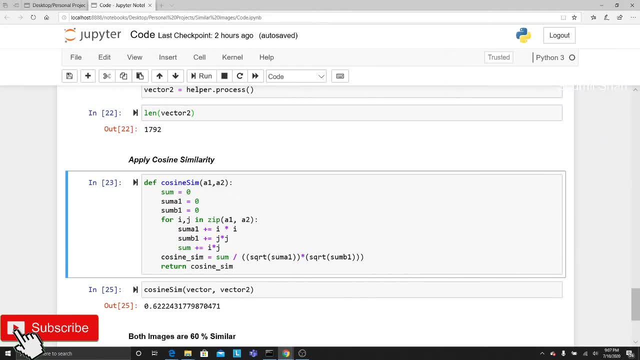 images. it's going to take time if you perform cosine similarity on all the vector, because you will basically go through all the images, gonna compute the cosine similarity and then at the end you would say, oh, which are the images who are matching certain criteria? so that search would 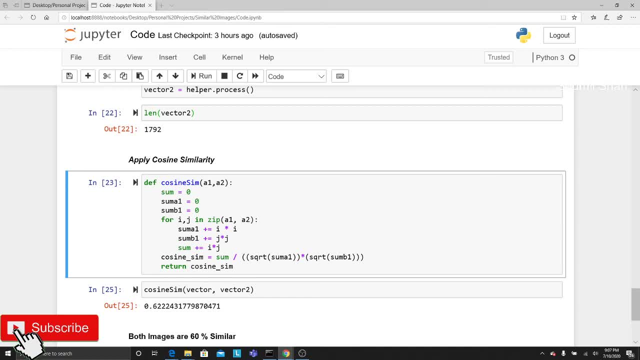 take a long time. so instead of doing that, i would recommend using elastic search for that kind of approach, because elk stack can do can perform search nearly realistically and it's going to take a long time to do that. so i would recommend using elastic search for that kind of approach, because elk stack can do can perform search nearly realistically. 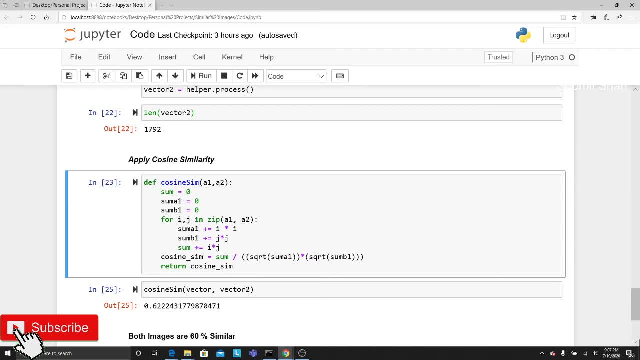 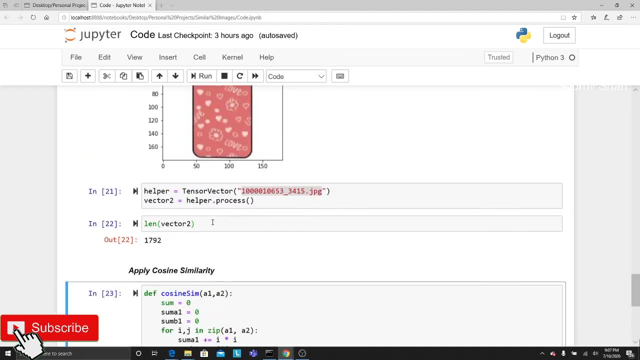 time, i would say because, um, as you know, i have been creating a lot of contents on elk stack. so for these kind of purposes, this is what elk stack is made for. so i would encourage you guys to try it out. i would at least say: try this out how, how basically the cosine similarity work, try.